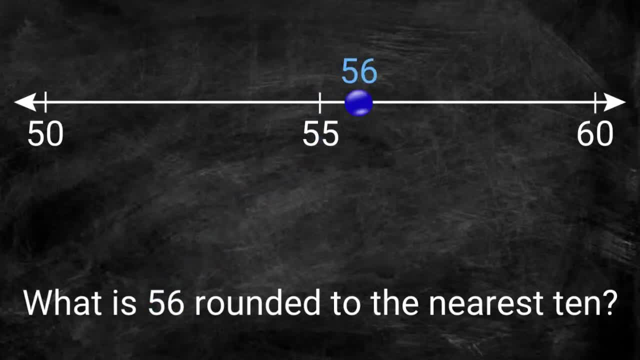 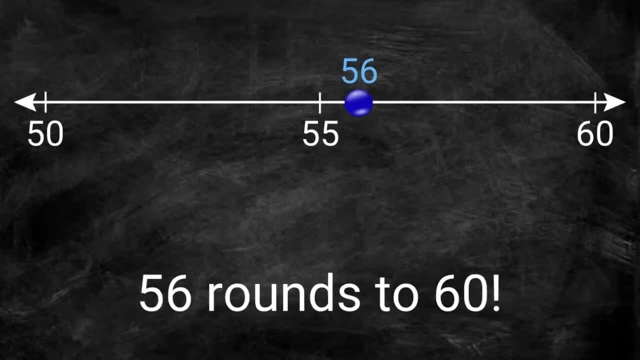 56 is located one space after the 55.. We can see now that 56 is located one space after the 55. That 56 is closer to 60 than 50. This means that 56 rounded to the nearest 10 is 60.. Look at this number line. Find the number 23.. Which 10 is 23? closest to 20 or 30?? 23 rounded to the nearest 10 is 20.. 23 is closer to 20 than to 30.. What is 89 rounded to the nearest 10?? 89 rounded to the nearest 10 is 90.. It is closer to 90 than 80.. This next one is tricky. What is 45 rounded to the nearest 10?? 45 actually rounds to 50.. 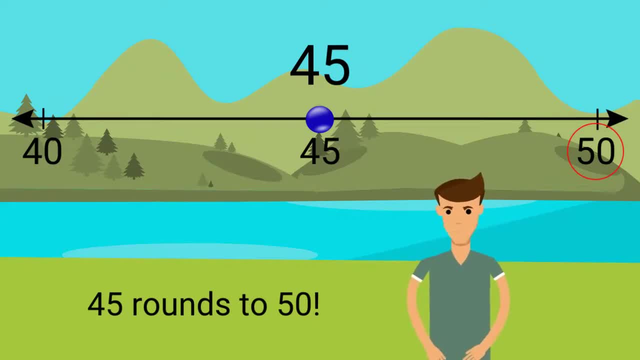 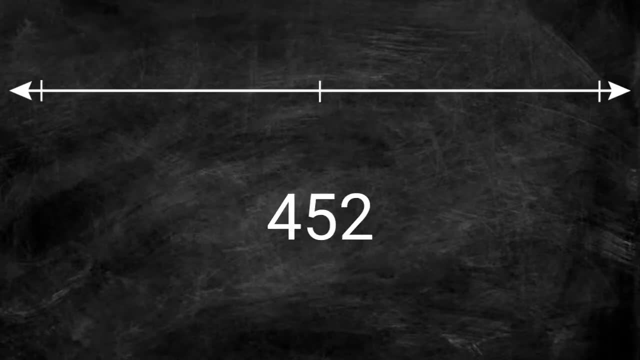 If the number is halfway on the number line always round up. Now let's get a little more challenging. Let's round 452 to the nearest 10. We see that the number 452 is really 4 hundreds, 5 tens and 2 ones. 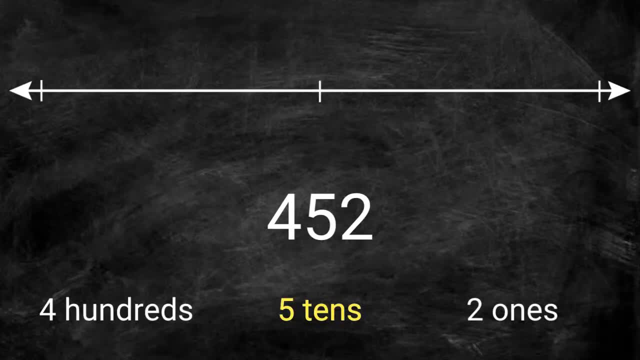 Since we are rounding to the nearest 10, let's focus on just the 5 tens. We know that 450 is the 10 lower than 452.. We also know that 460 is the 10 higher than 452.. 455 has to be exactly in the middle. 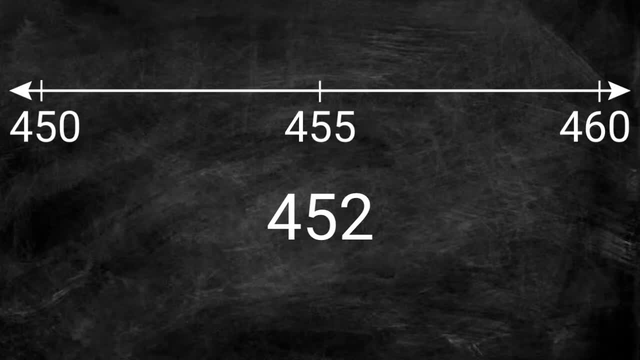 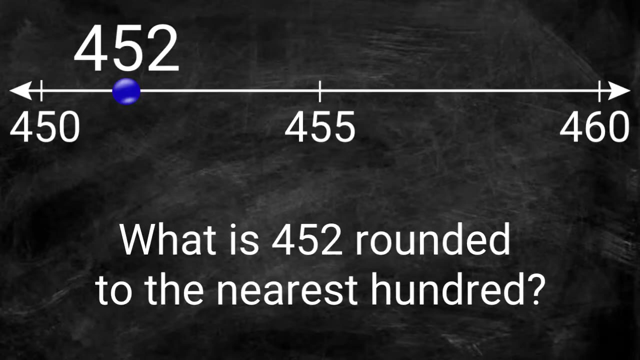 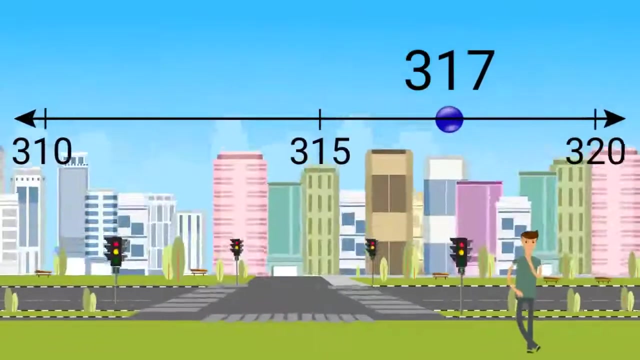 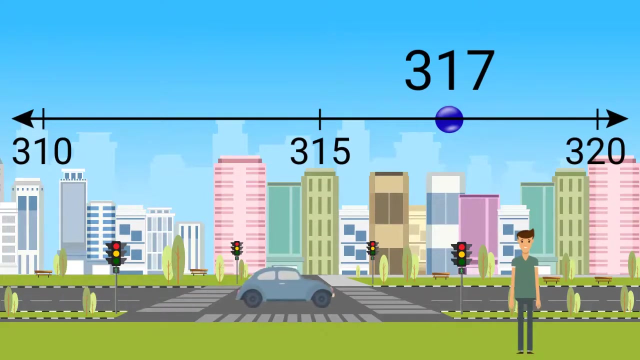 Where should we place 452? 452 goes right here. Now we can round 452 to the nearest 10.. Does it round down to 450 or up to 460? 452 rounds down to 450.. What is 317 rounded to the nearest 10?? 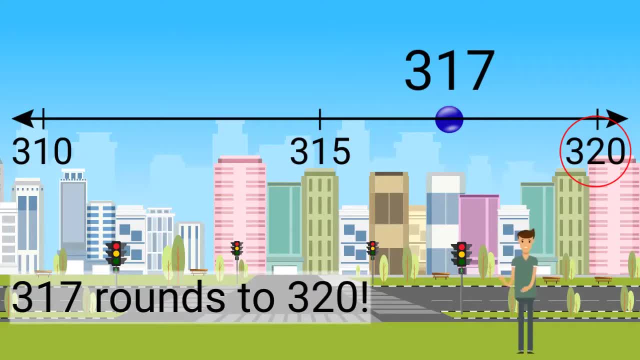 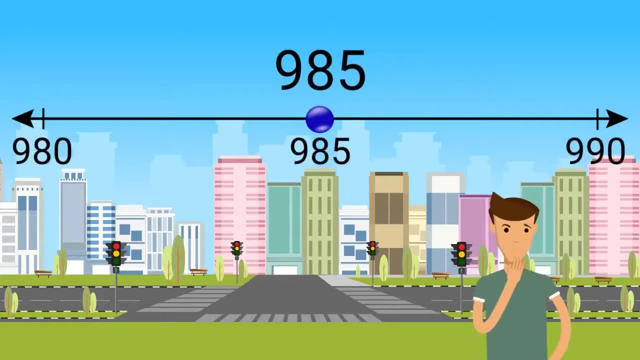 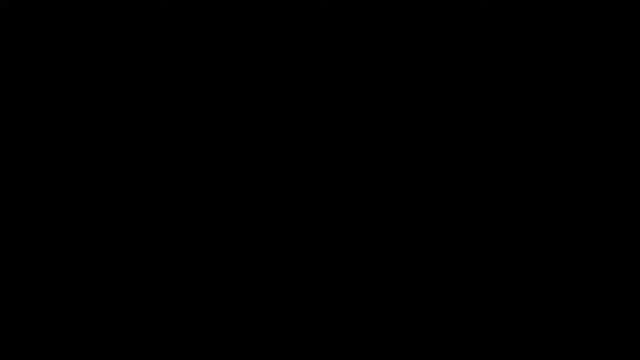 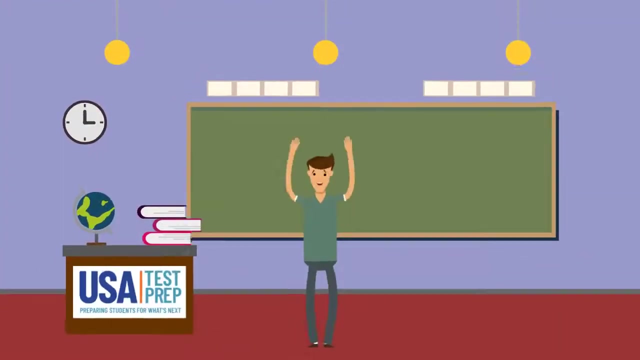 317 rounds up to 320.. 317 is closer to 320 than 310.. What is 985 rounded to the nearest 10? 985 rounds up to 990.. Remember numbers that are exactly in between always round up. That was a lot of learning we did today. 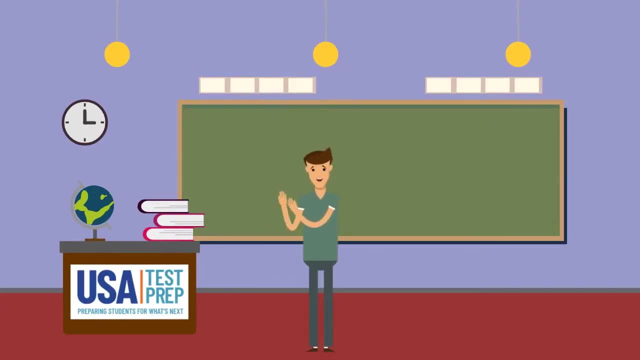 Making a number line to help you round numbers is a great strategy. Make your own number lines to help you see whether to round up or round down. See ya, and keep learning.